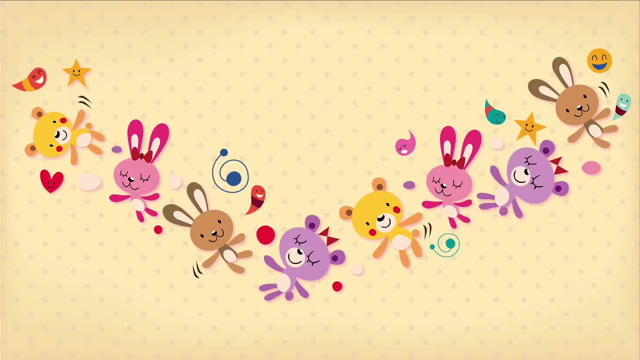 I know it seems really easy when you say it doesn't it? But it can be quite a hard thing to do. So let's try some stuff and see if we can make being still something we're really good at. You can have your eyes open or closed for this. 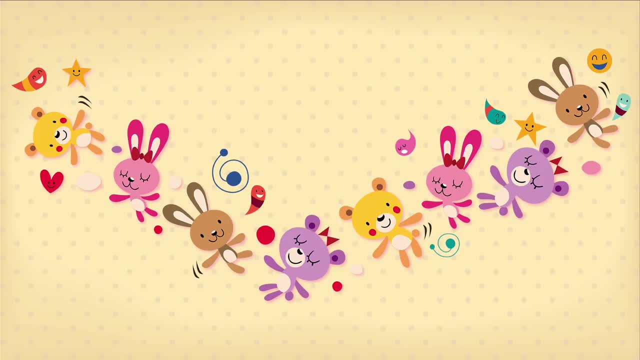 You decide what works best for you right now. The first thing that will help us is to know the difference between moving, sitting and being still. I bet some of you are really good at playing musical statues or freeze dance, so you know you can be still when you're playing a game. 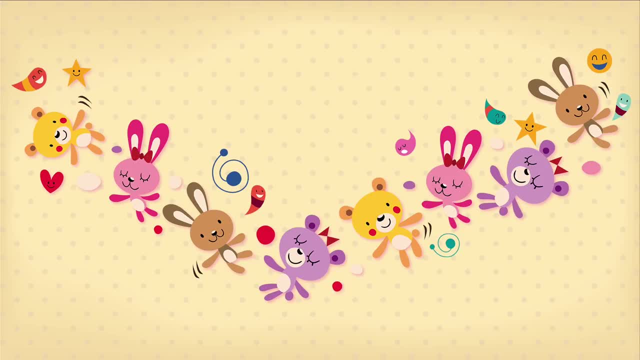 Let's try and play something similar now in our peace out position, exactly where you are. Let's call it wiggle flop. It's different to the party game because in wiggle flop you don't go stiff, you go soft, like a sleepy cat. 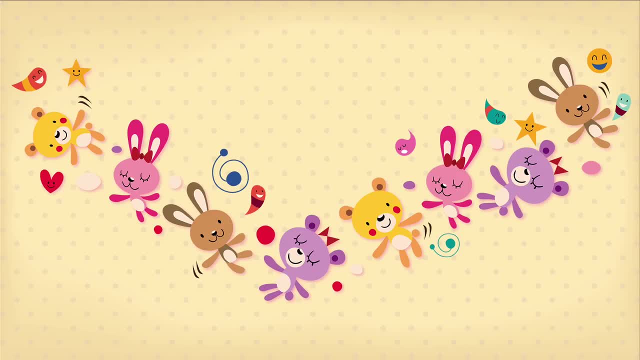 All still soft and floppy, as can be. When I call out flop, that's when you stop and go: really floppy and still Are you ready, Ready? Okay, Wherever you are, see if you can start to wriggle. 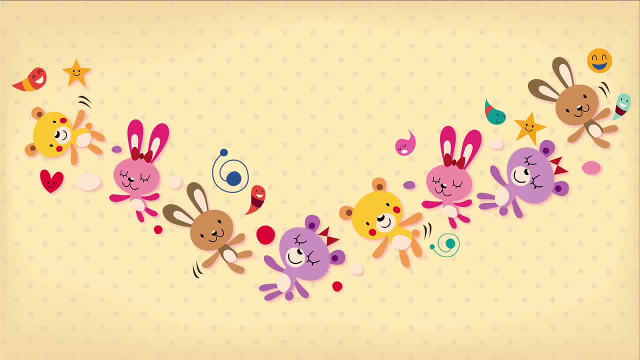 Wriggle your legs, your arms. jiggle your fingers, your toes. Can you wriggle your body too? Yes, your chest and tummy and your face, your nose and mouth, everything wriggling and jiggling. 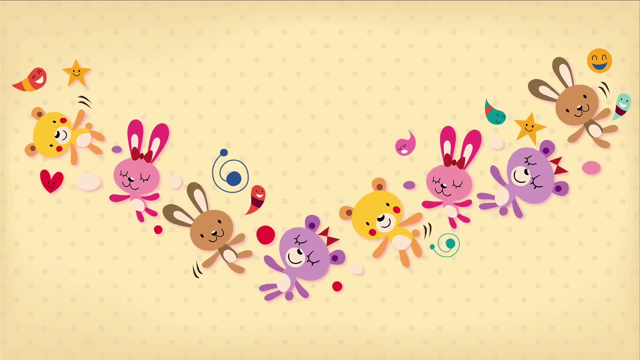 That's it. Keep going Wriggling, a little bit more Wriggle, wriggle, wriggle And now flop. Totally droopy, No moving, Not a sausage, Really heavy and floppy. Remember to breathe. 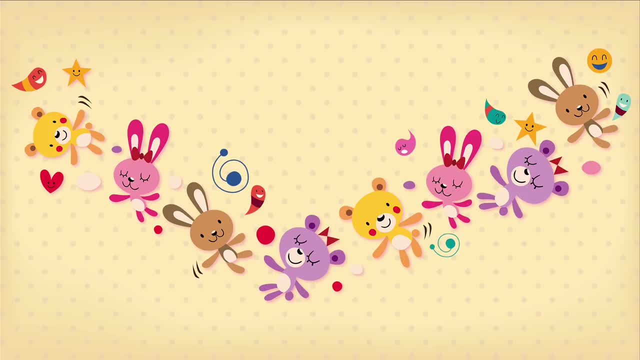 Breathing is definitely okay in wiggle flop, And now let's wriggle again. Yeah, get those legs and arms going, Your feet and hands, your fingers and toes, all the wriggles moving up into your body and head. 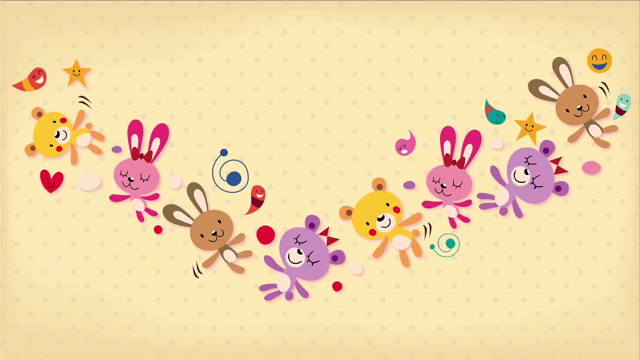 Every last part of you having a good old fidget, That's it. A little longer. Wriggle, wriggle, wriggle And flop. Like you've been switched off. Everything flopping down, Not a big deal. 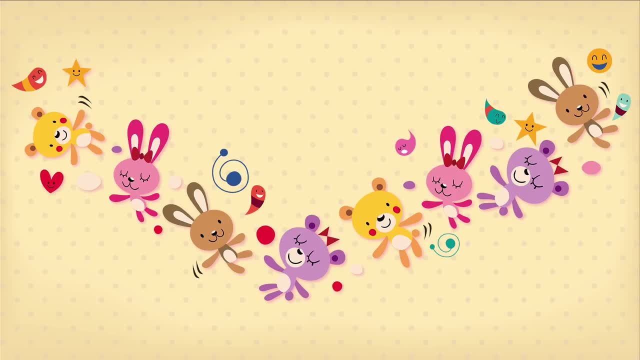 Not a flicker or flutter- Breathing, yes, but total, relaxed, droopy stillness. I reckon you might be pretty good at this. In fact, you could be getting better with each time we play. Okay, let's have one final go. 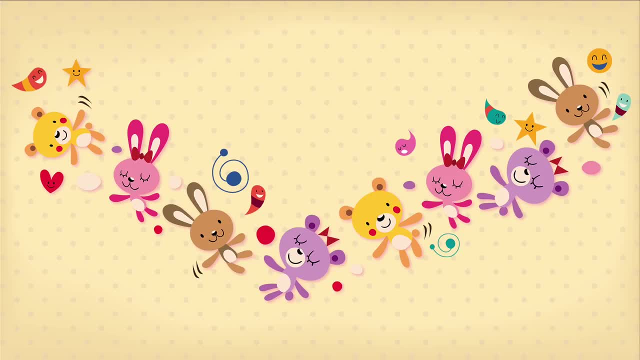 And this time see if you can really enjoy your flop time at the end. Let's get wriggling. Get those legs going And those arms. Yes, now your hands And feet, Fingers and toes, Body and face. 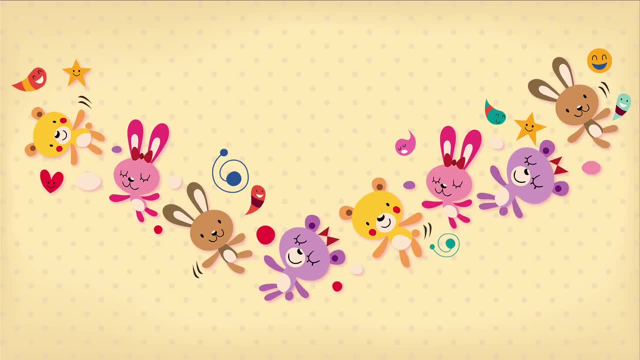 That's it, The wriggliest you've been for ages. Like you're the wriggle champion of the world And flop, All the wriggles melt away And you're as still and relaxed as can be. You get the gold medal for floppiness. 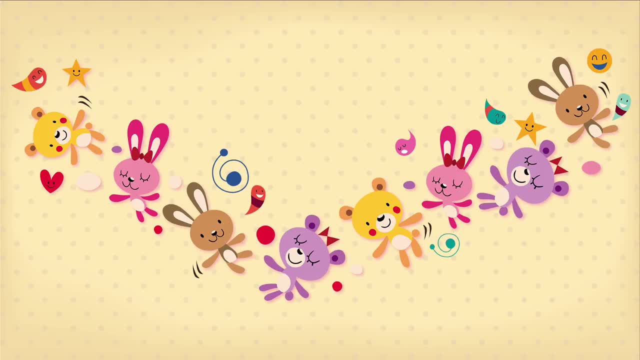 Breathing and enjoying the feeling of being so heavy and still Feel it in your body. How your arms feel. now Your legs too, What real stillness, with no holding or tension, feels like in your body. Notice how your fingers and toes feel too. 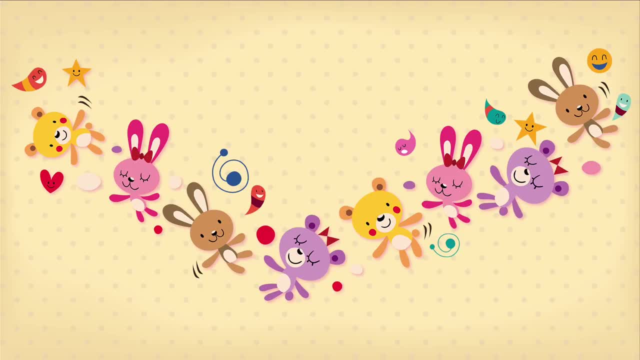 All these parts of your body almost tingling because they are so floppy and relaxed. Well done, It's time to return. Listen to the sounds around you, Notice where you are lying or sitting, Feel where your body meets the chair, ground or maybe bed beneath you.